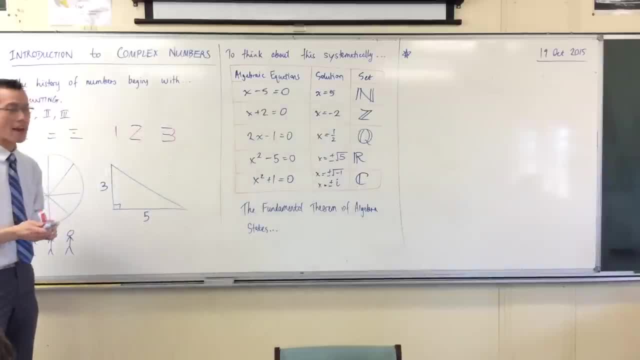 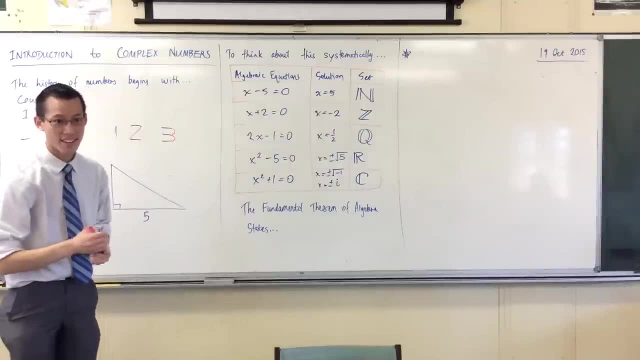 They are more than just the real numbers, They are bigger than that. Now here's what's really profound, and I'll answer this question: Yeah, no, yeah, Oh yeah, I was just wondering if they're part of complex numbers. 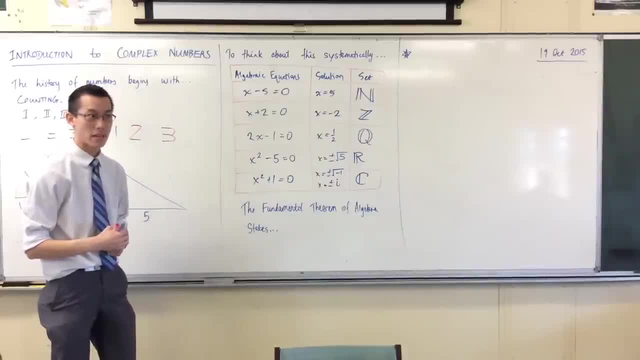 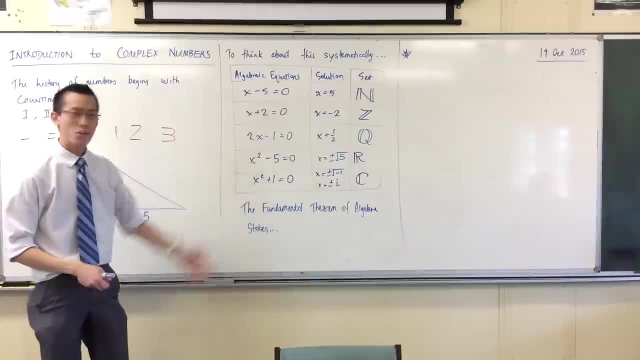 are there other numbers that are not like imaginary, But not super complex? Yes, yes, I'll talk about that in a second. okay, Now here's the really really cool thing. This is why my table has this many rows and no more. 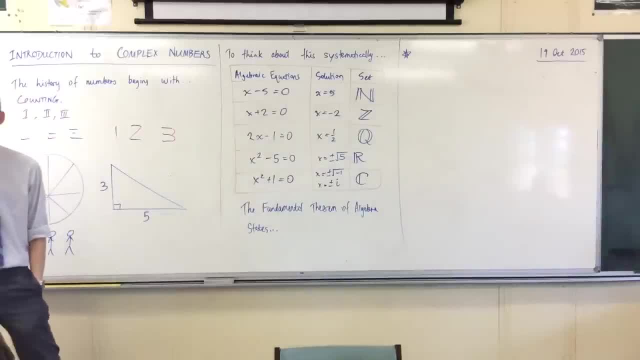 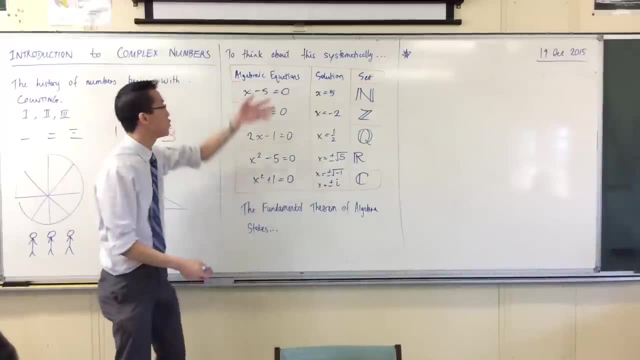 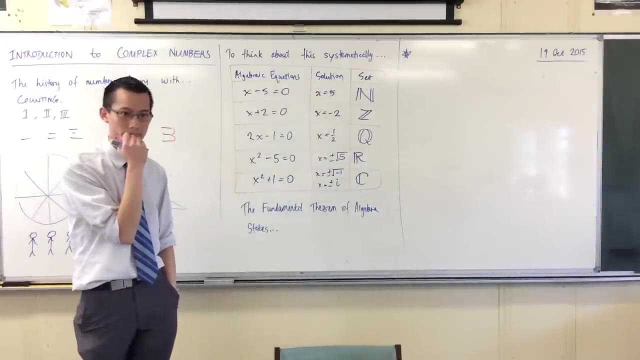 If what you're doing is trying to arrive at numbers by means of algebra and counting numbers, if these are your building blocks and these are your building tools, okay, this complex numbers. these are the end of the line. There is no other kind of number. 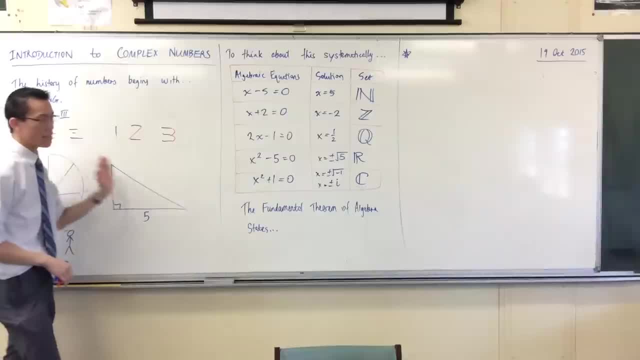 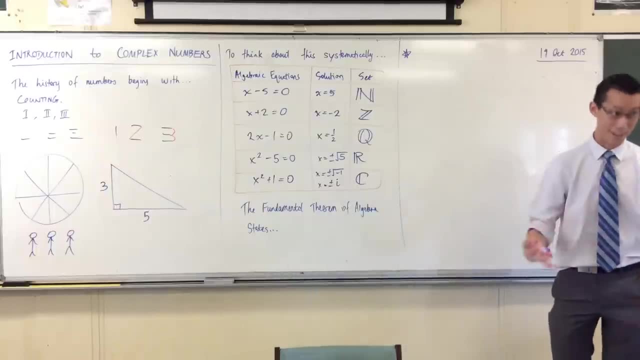 Then you can combine plus, minus times, divide and counting numbers. There's nothing else you can make out of this. In fact there's this big- you can look it up later- important theorem in mathematics called the fundamental theorem of algebra. 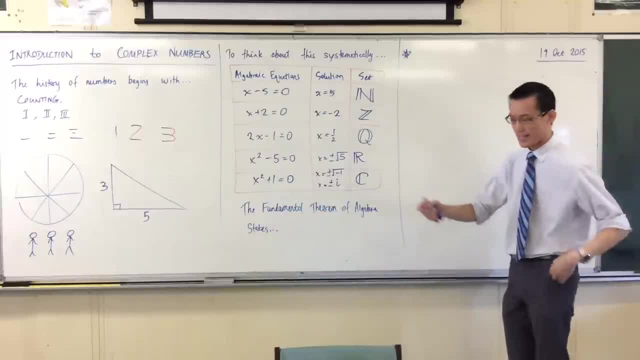 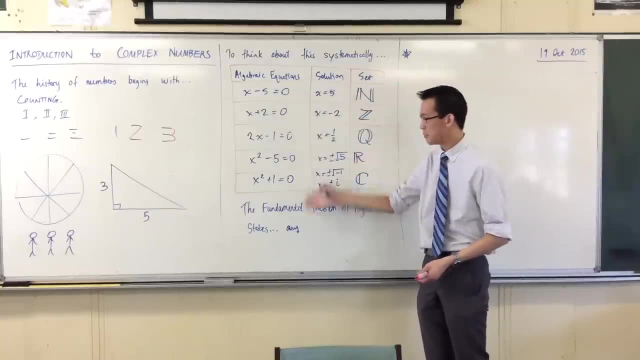 You know, something's really a big deal when they say fundamental, What it states is that any polynomial. so you see, these are all polynomials. I mean, admittedly, these are very simple ones, They're just linear, but I could make them more complicated if I wanted to. 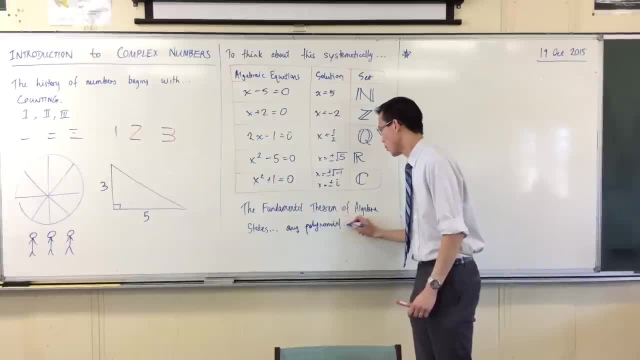 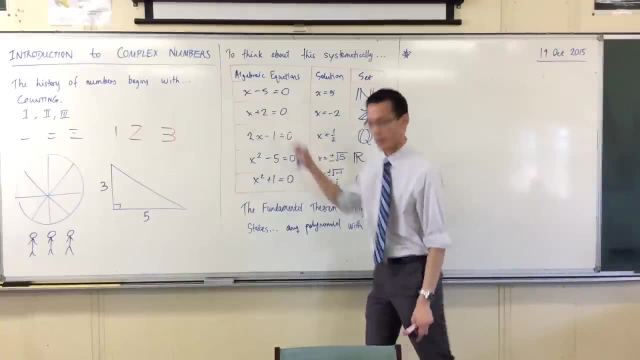 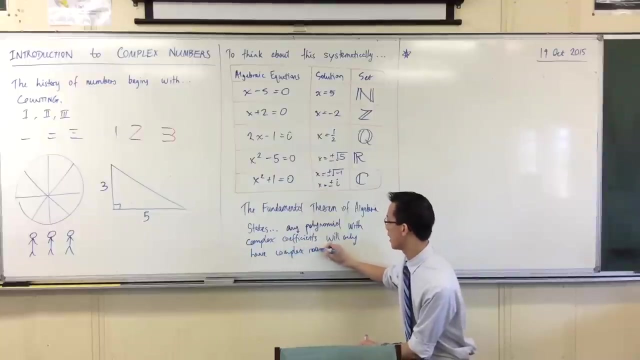 Any polynomial with Complex coefficients- so that's these numbers in here. right these numbers out the front- Any polynomial with complex coefficients. it will only have complex roots. This is the end of the line. Unlike every other kind of number. 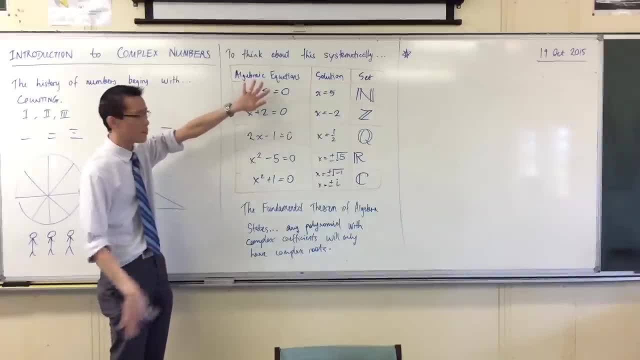 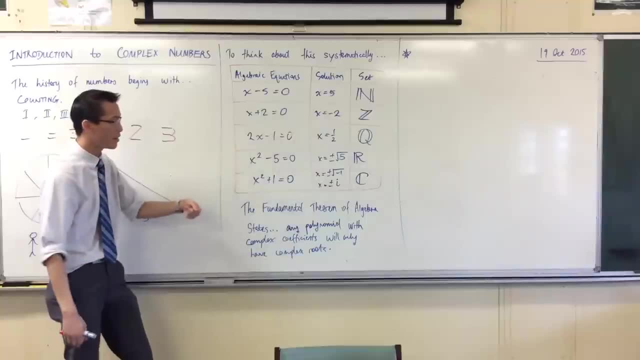 For instance, you can make an equation with just counting numbers, but its solutions are not counting numbers- Right, they might be rational numbers. You can make an equation with irrational numbers- right, and its solutions will not be rational numbers. They'll be something else. 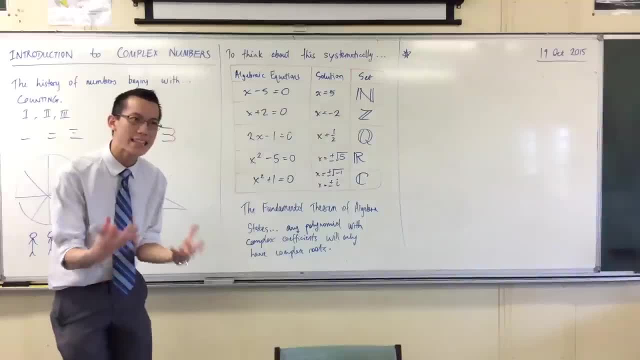 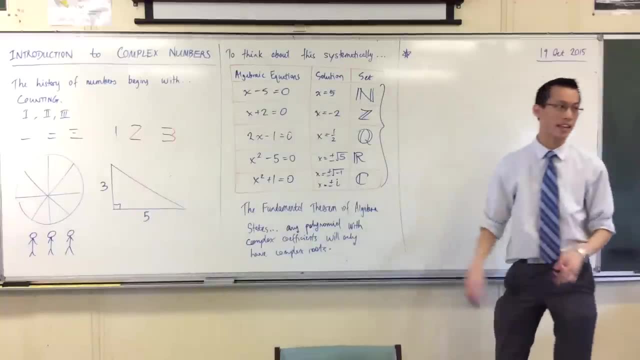 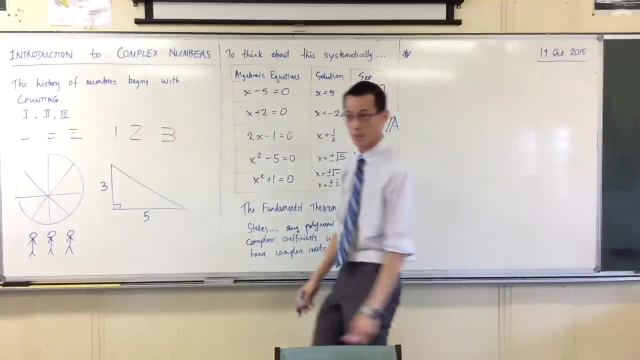 But once you get to complex numbers, you can't make anything more right? There's another fancy phrase for this. Firstly, by the way, all of these guys, all of these sets belong to, because they were built by algebra. they're what we call, imaginatively, the algebraic numbers. okay, 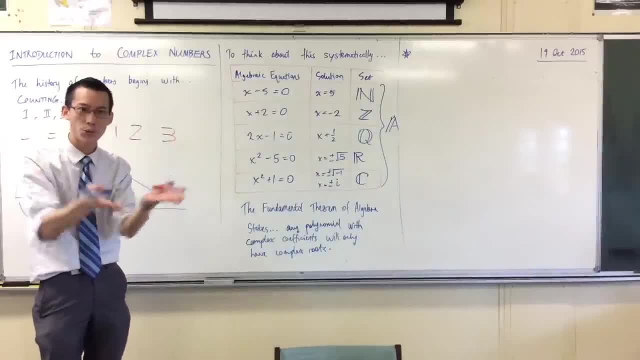 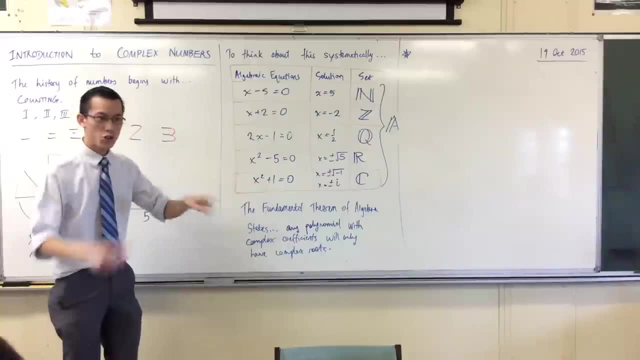 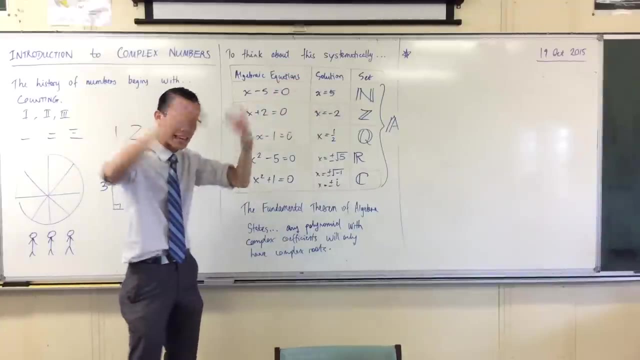 The complex numbers are what we call an algebraically closed set. Algebraically closed Meaning that when you construct equations with these complex numbers, you can stay. the answers stay within the complex numbers, Whereas I can create equations with other kinds of numbers and get out of there. 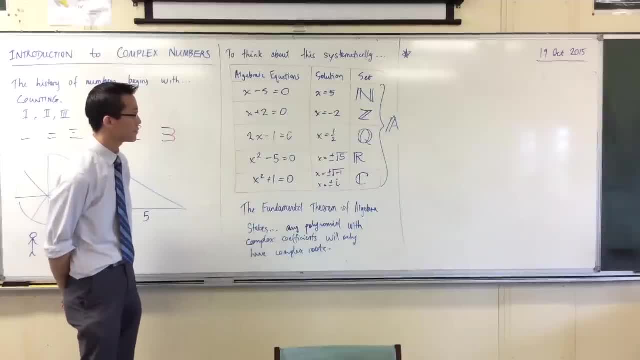 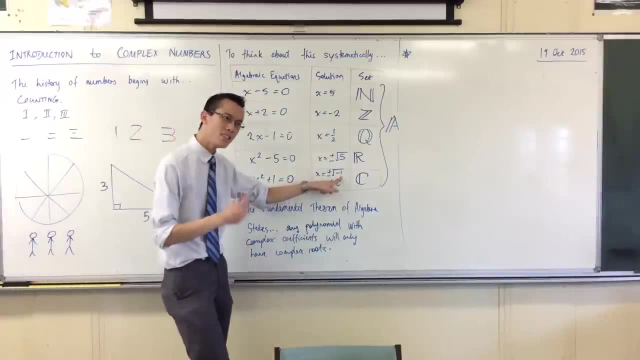 All of these are made with counting numbers, right? Okay, so this fundamental idea that I can have a negative number underneath the square root and it isn't just like meaningless, I can just ignore it, okay. Actually, it's something that I can work with. 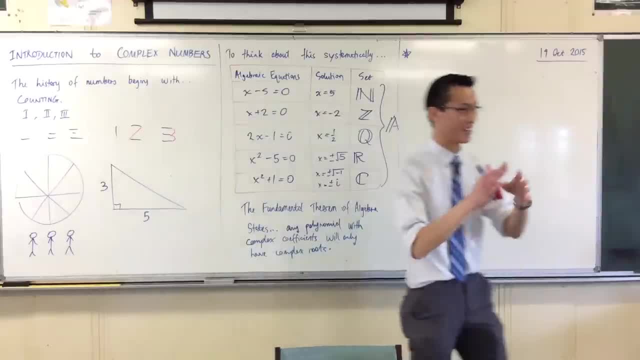 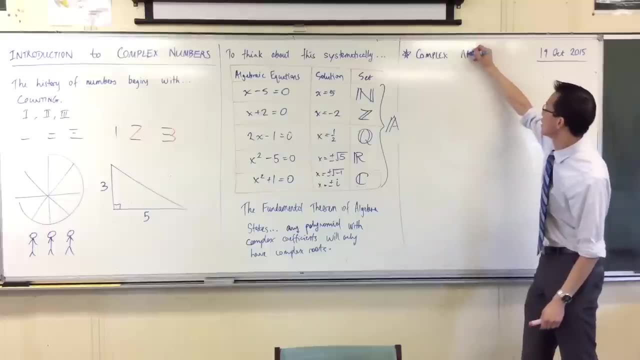 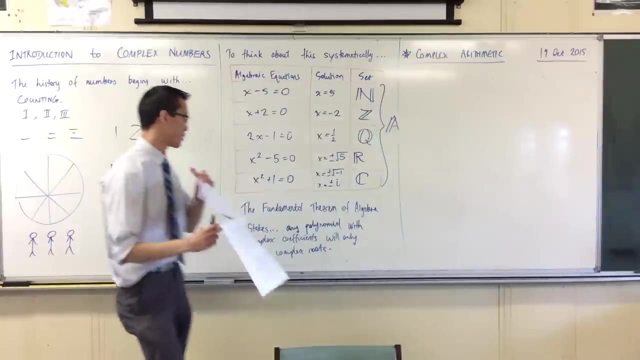 That's the basic assumption we're going to run with, and it's going to be one heck of a ride. okay, So new subheading: complex arithmetic, As it turns out, complex numbers. despite how weird they sound like, you can't do operations- sorry, you can't do measurements on them. 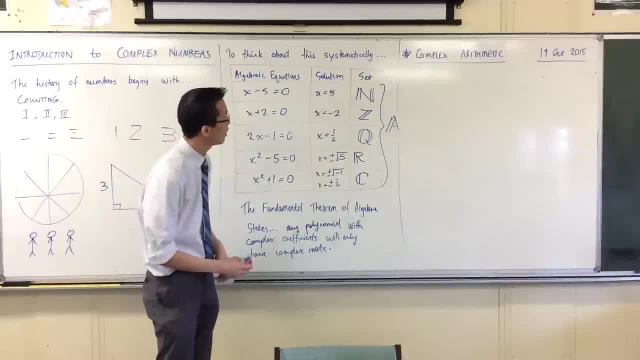 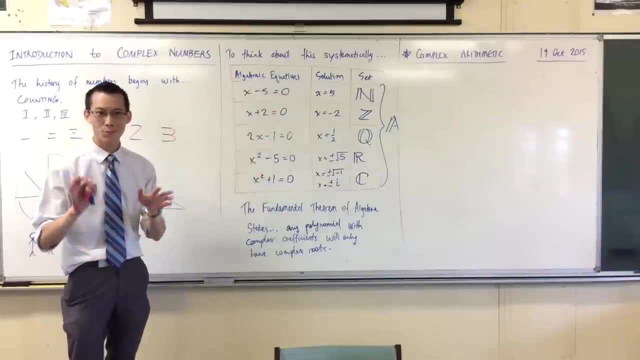 like: oh, how far is i? centimeters? It doesn't quite work like that. We can do operations on them just like we can with any of the other numbers. okay, With some interesting other conclusions. In the same way that you know all the rules, you know. 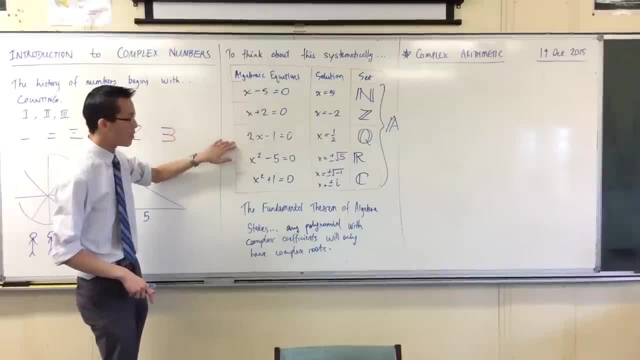 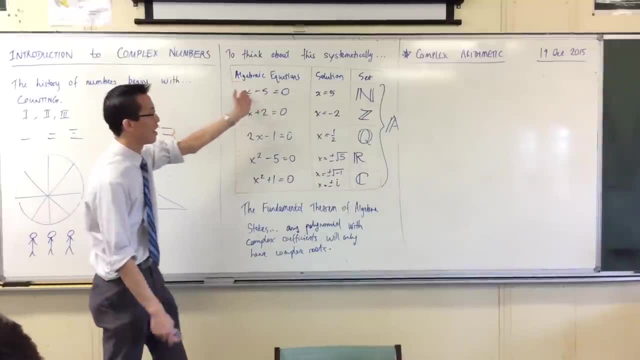 for normal counting numbers, rational numbers etc. they apply to irrational numbers, Sort of right. So, for instance, if you multiply together two counting numbers, like say two times three, right, That's the same as three times two. 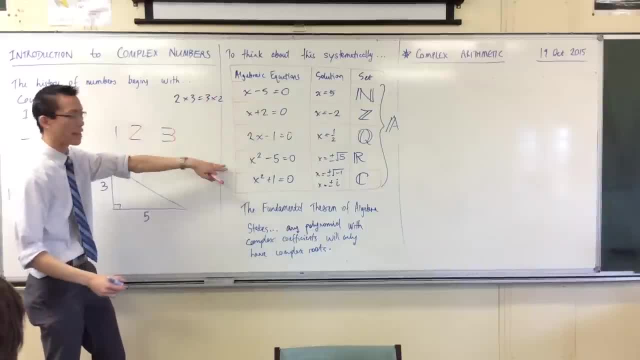 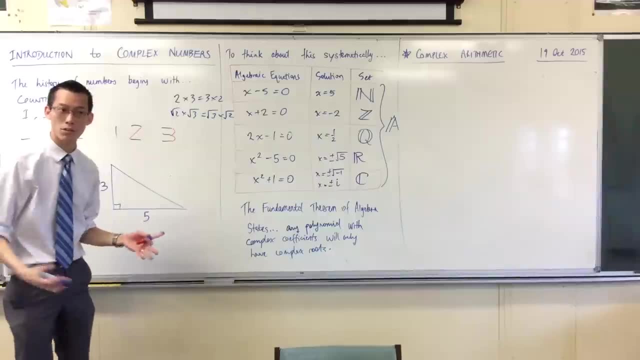 You agree with that right. And if you take- you know, thirds, you can say the square root of two times the square root of three, that's still the same as the square root of three times the square root of two. So these rules apply. 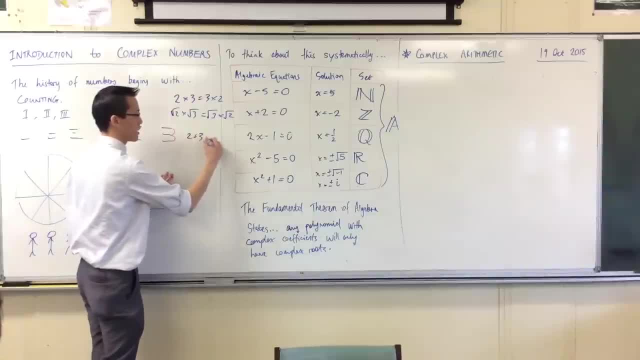 But not all of them apply, right. For instance, two plus three is equal to a number, right- five. But the square root of two plus the square root of three doesn't equal the square root of five, right, Because something different is happening with these numbers. okay. 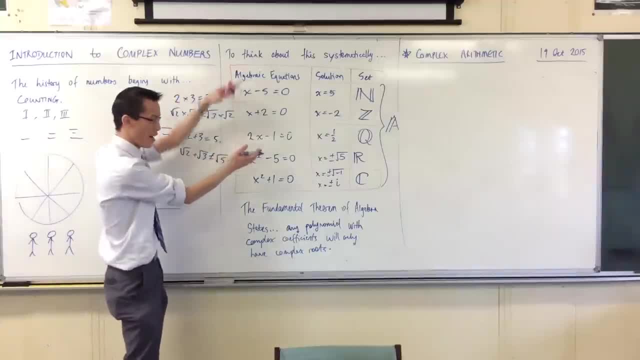 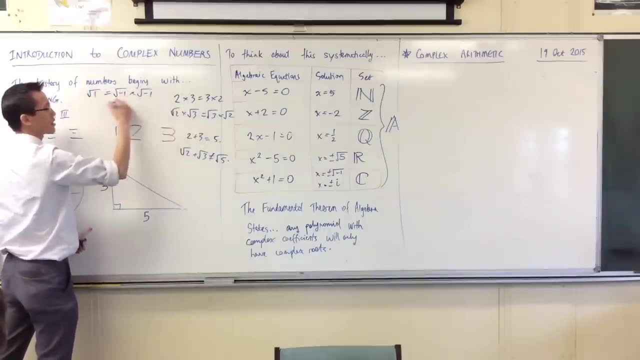 So we can't simply take anything right. We can take everything that we know and apply them here, As you will see. let's quickly rehearse it. As you will see, things quickly start to break down if you try and do this right. 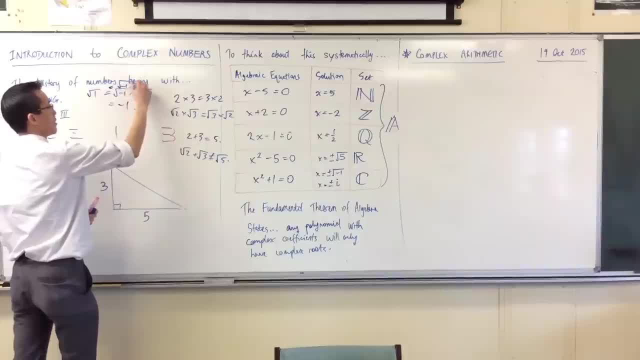 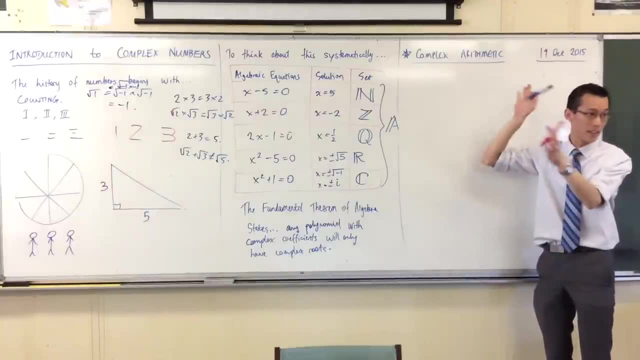 Oops, I skipped a step, sorry. Okay, so the rules apply, but they don't, And we have to be a little bit careful with them, which is why there's this whole idea, this whole other branch called complex arithmetic. okay, 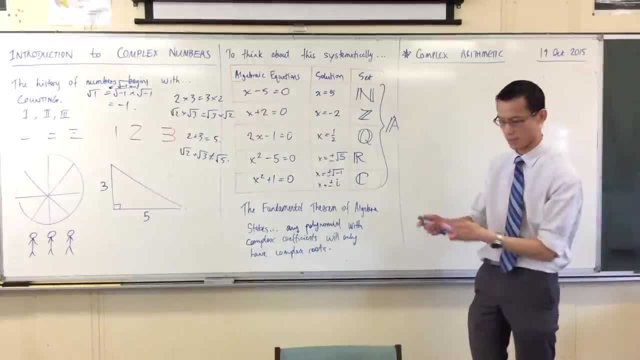 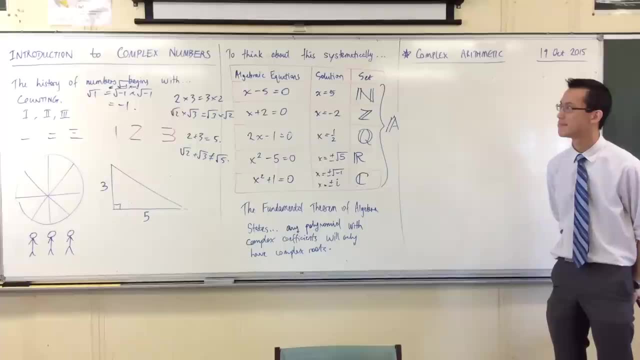 So first let's lay down some notation and some definitions. I need a new color. Yeah, Isn't that like half correct? Because the square root of one is also as close to minus, Ah, so okay. So in case you wanted to know, right? 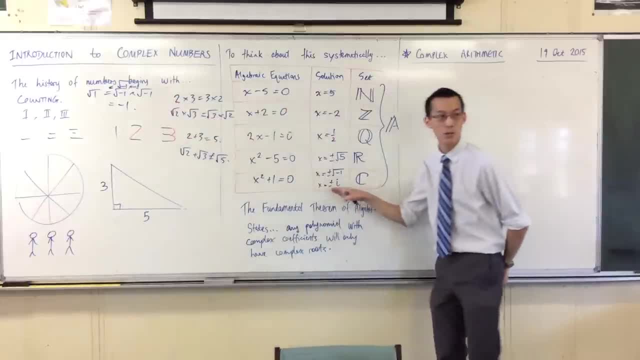 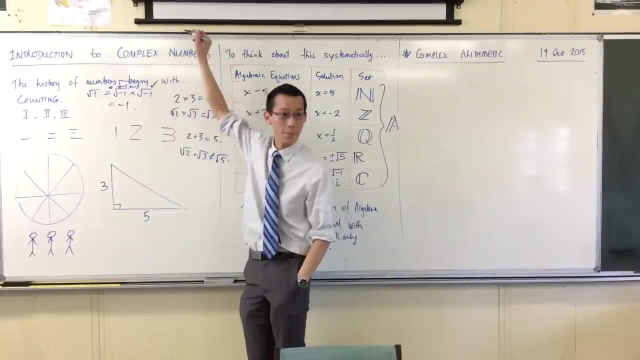 the reason why this is starting to break down is because we are walking into complex territory here. One is equal to minus one times minus one. That's okay, right. The square root of negative one times the square root of negative one really is negative one. 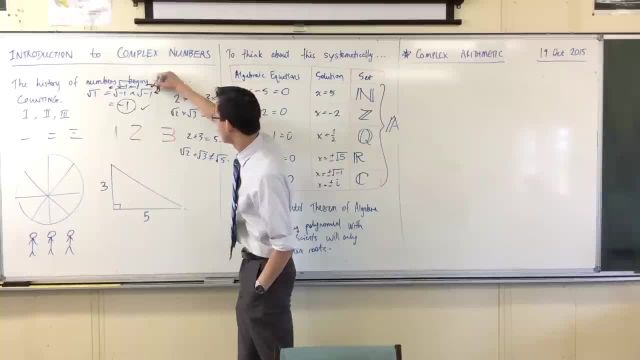 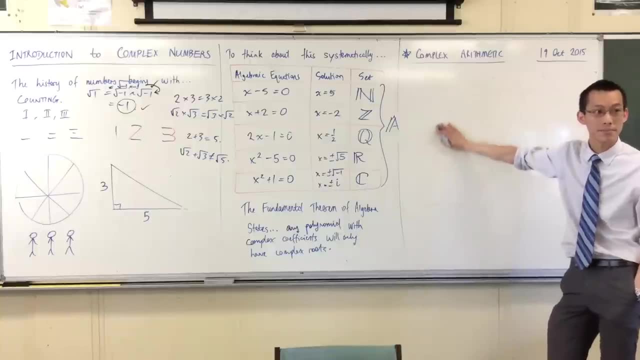 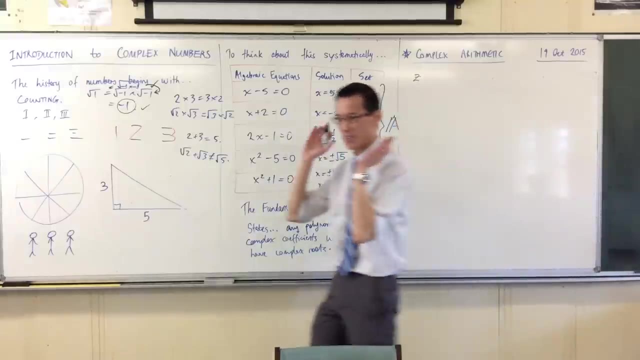 That's okay. Where the problem is is here. Now the question is why, And we will get to that as we unpack complex arithmetic a little bit further, Okay, Okay. so here we go, Let's start. I'm going to introduce to you the basic number. 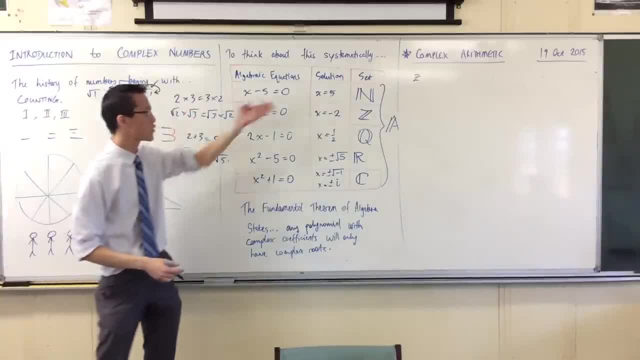 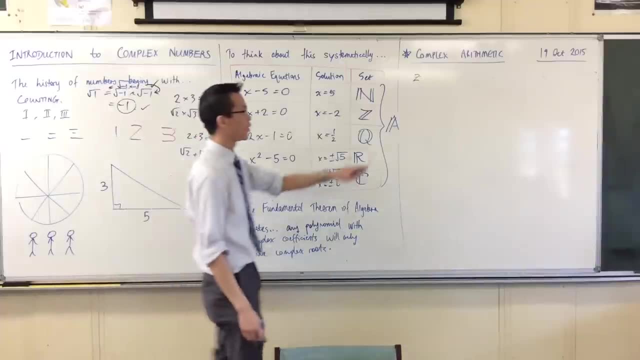 the basic pronoun we use for indicating all complex numbers. Just like when you've got an unknown in real numbers, we use x. When you've got an unknown and you're in complex number land, we use z. I am going to highly, highly encourage you. 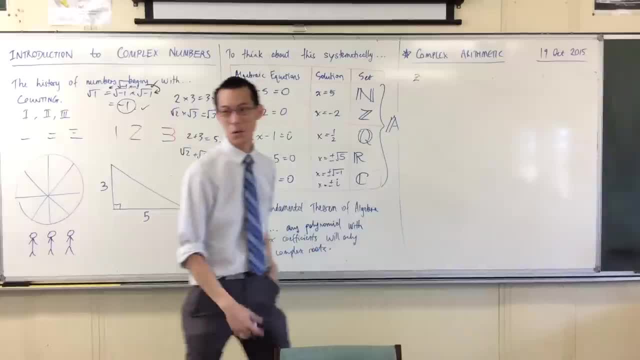 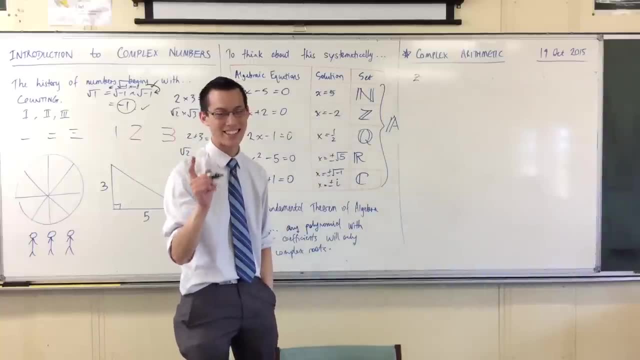 highly, highly encourage that you put a dash through all of your z's so you do not think that they are twos. okay, Believe me, you only need to lose one mark to realize why do I write my z's like twos. 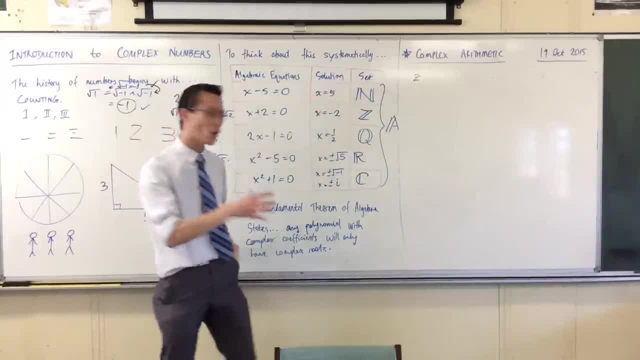 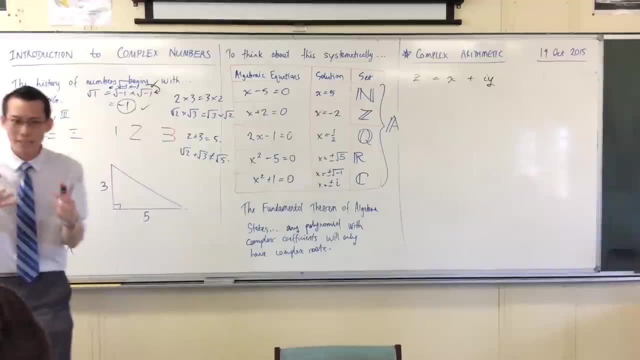 Just save yourself the trouble and put a dash through it, okay, So complex numbers are in this form: x plus iy. What does that mean? X is that real number, just like you've been using real numbers before. It can be positive, negative, rational. 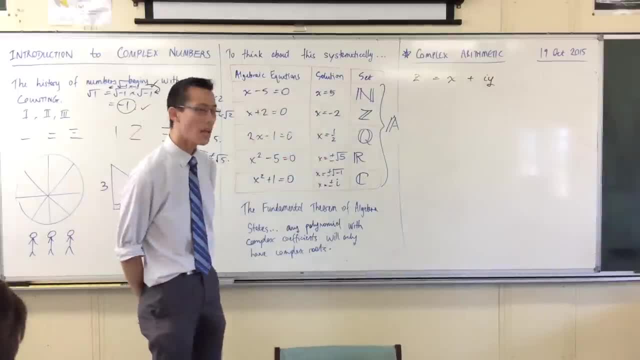 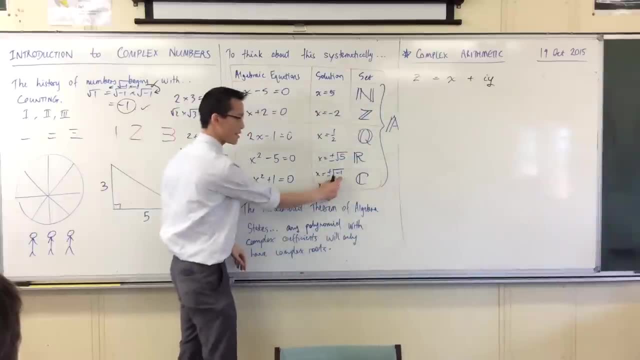 A square root. that's all fine. Then you've got, in addition to this real part over here, you've got a part which is a multiple of this guy right, A multiple of the square root of minus one. Now, when I first started learning about complex numbers, 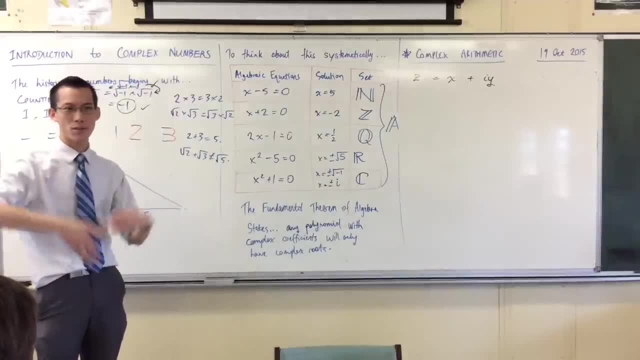 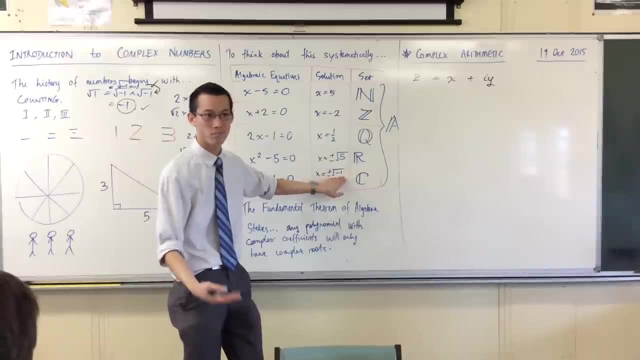 I was like: why square root of minus one, Why not square root of minus two or minus three or whatever? And the reason why is because everything is a product. every imaginary number is a product of the square root of minus one, For instance, the square root of negative two. 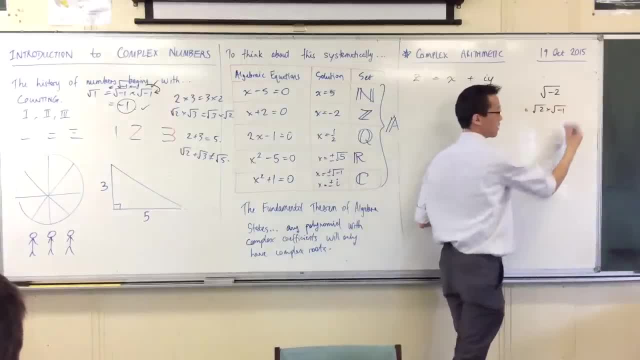 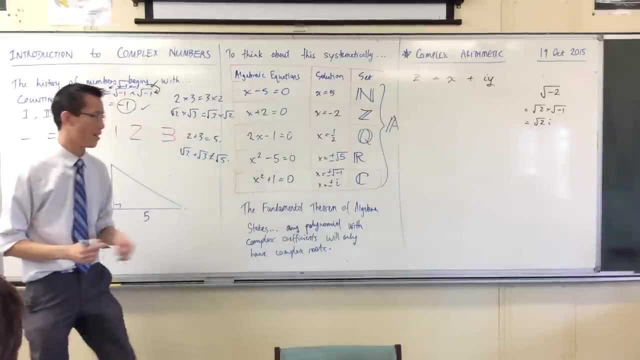 is really just the square root of two times the square root of minus one. That's actually okay. So this is the square root of two times i, So I can write every square root of a negative number in terms of this one. So this is like a fundamental piece, if you like. 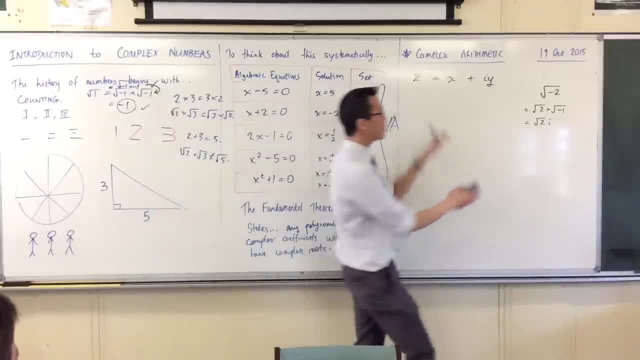 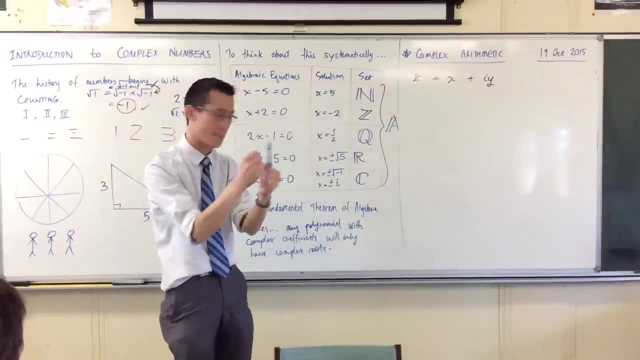 So let me get rid of that, because I'll need that space. I've got a real part and I've got this part over here which is imaginary. You've got two pieces to it and they don't mix together. They're a bit like when you've got a number. 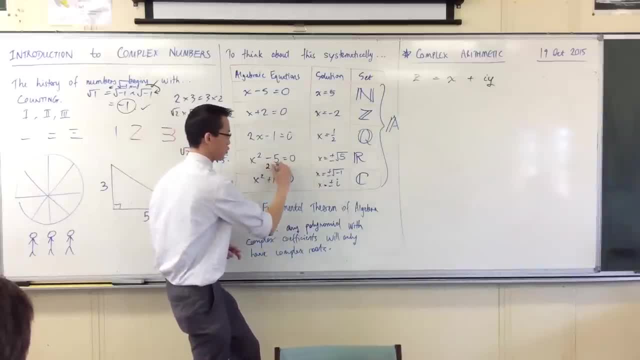 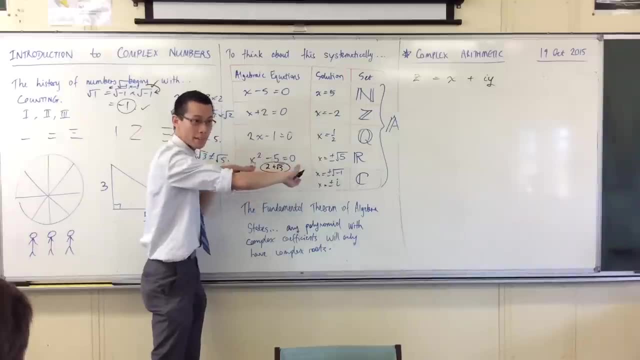 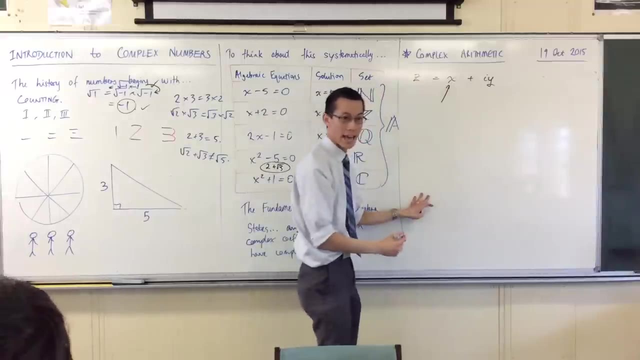 let's go back in irrational land. If I had two plus root three, this is an irrational number. But I can't mix those bits together. they stay apart. they're like oil and water, Just like this real and imaginary bit. So we call this guy the x. 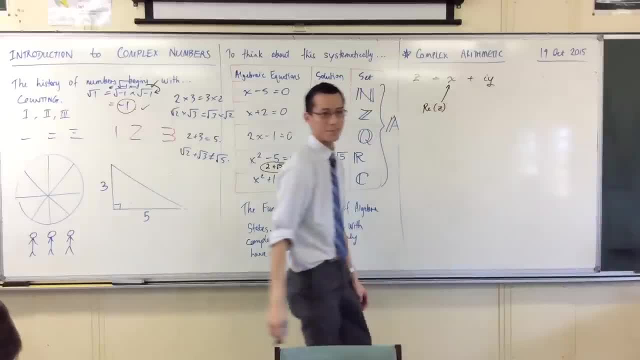 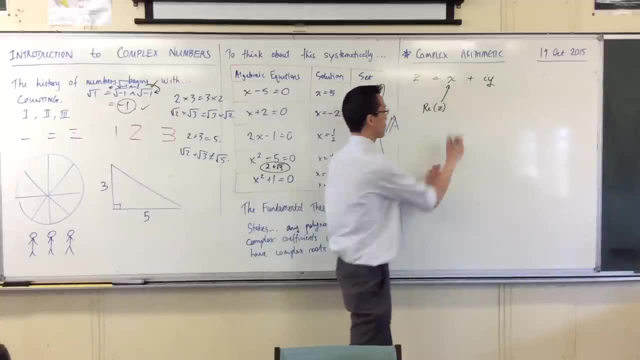 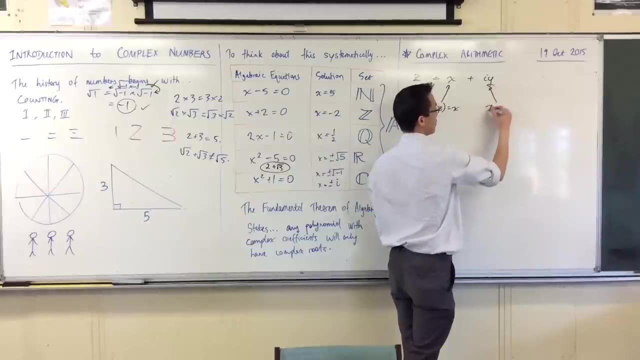 we call him the real component of z, Re being our abbreviation for real. The real part of z is just x. It's equal to x. Okay, Otherwise there's an imaginary part. this part, The imaginary part of z, is just y. 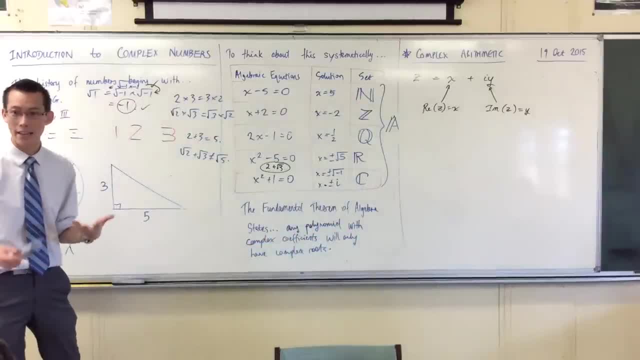 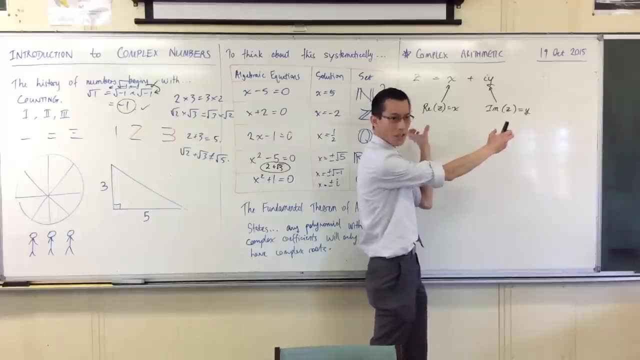 So it's the size of the imaginary part. it doesn't include an i in it. Yeah, it's like the magnitude of it, Now being that you've got these two parts and they're separate to each other. that's why z, despite being one number, 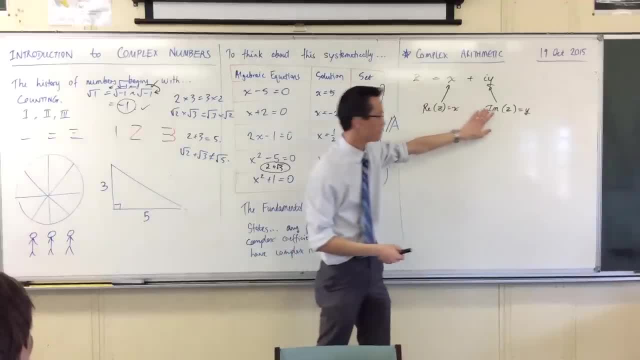 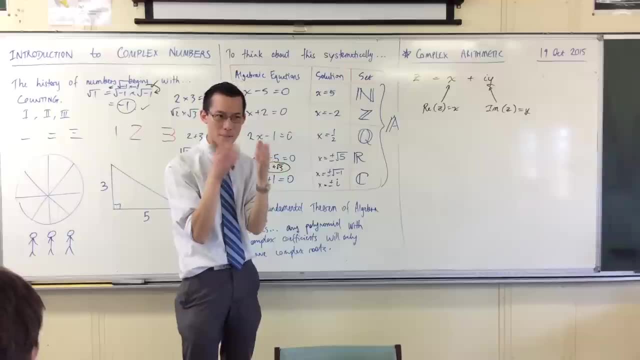 he's one number with. he's not just simple, he's got complexity to him, hence complex numbers. All they mean is there's more than just a simple number going on here. There's two parts to it, Okay, So a little bit of extra language here.